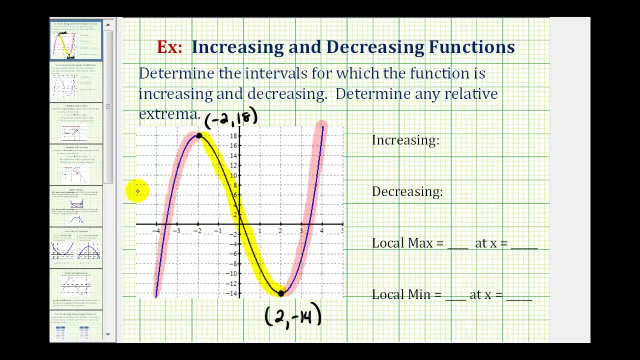 and therefore it's increasing. Notice how the function is decreasing on. this interval changes from increasing or decreasing at x equals negative 2, and then from decreasing to increasing at x equals positive 2.. The last thing to remember is, as we move right on the x-axis, we approach positive infinity As we move. 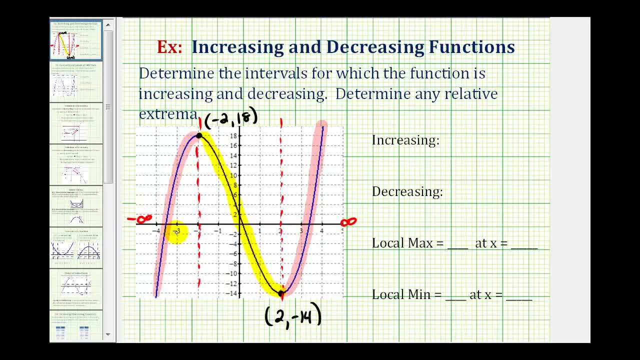 left we approach negative infinity. Now we have all the information we need to determine where the function is increasing or decreasing and list any relative extrema. The function is increasing from negative infinity to negative 2, so we use intervals on the x-axis to determine where the function 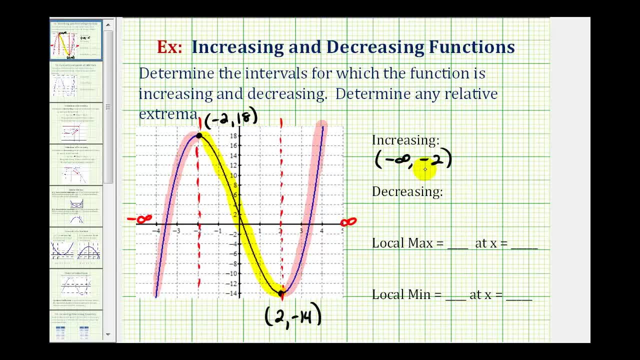 is increasing or decreasing And we're not going to include negative 2 in the interval, because at negative 2, the function changes from increasing to decreasing and that's where the relative maximum occurs. But the function is also increasing on the interval from 2 to infinity, again not including positive 2.. 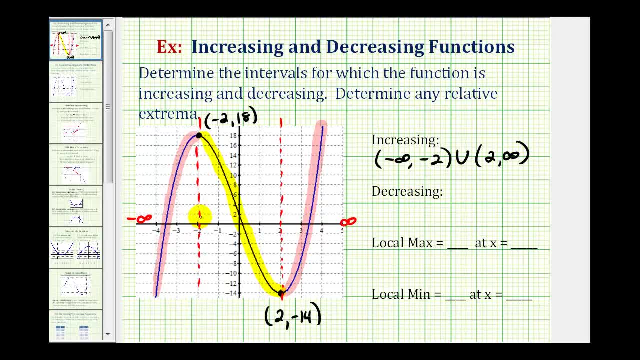 Then the function is decreasing on the open interval from negative 2 to positive 2.. This high point represents a relative maximum, which we can also call local maximum, And this low point represents a relative minimum, which we can also call a local minimum. So the local maximum is equal to the function. 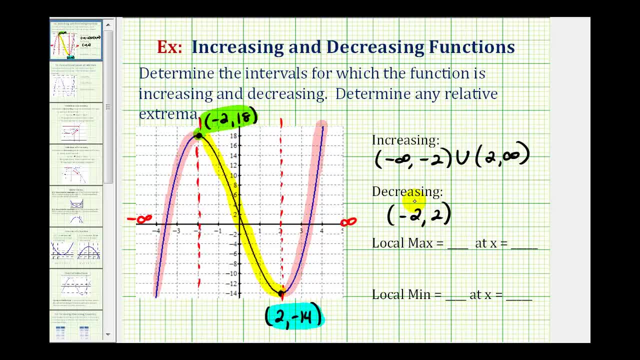 value or y value. So the local maximum or relative maximum is equal to 18 when x equals negative 2.. The local minimum or relative minimum is equal to negative 14,. the function value at the low point, at x, equals positive two. The last thing I do want to mention is you may be asked to express your intervals using 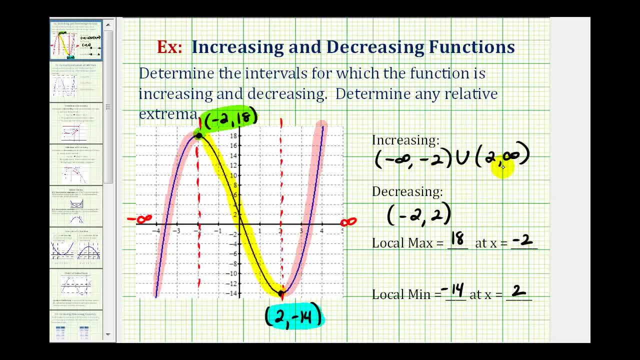 inequalities instead of interval notation. So let's go ahead and show that, just in case The interval from negative infinity to negative two would be x is less than negative two, or the interval from two to infinity would be x is greater than two, The open interval from negative two to two can be written as x is greater than negative. 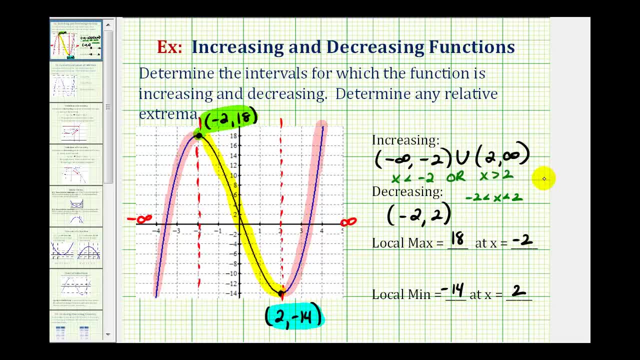 two and less than two, And I think we'll go ahead and stop there. I hope you found this helpful.